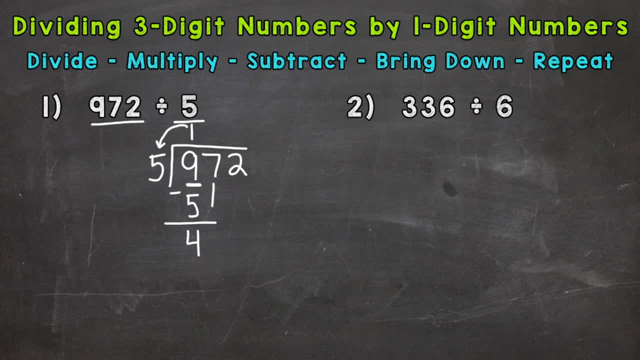 is 4, then we bring down. we bring down our next digit, that's 7, so we have 47, and now we repeat the process. so 47 divided by 5, how many whole groups of 5 out of 47. so think of your 5 facts. well, we know, 8 times 5 is 40. well, let's try. 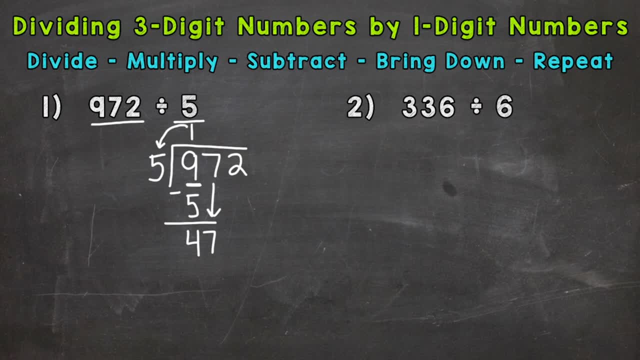 9 times 5. 9 times 5 is 45. so we can pull 9 whole groups of 5 out of 47. so we put our 9 here and then we come back around and multiply 9 times 5, 45, subtract, we get: 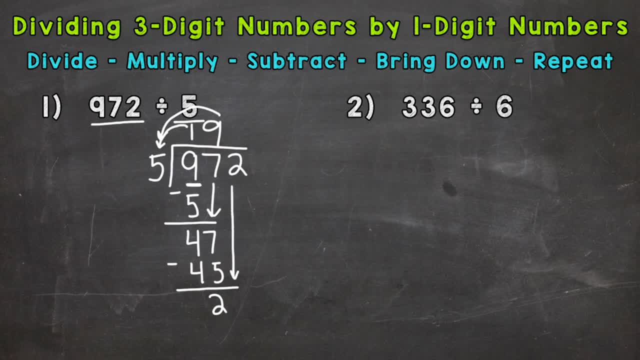 2 bring down. so now we repeat: so divide 22 divided by 5, so how many whole groups of 5 out of 22? well, 4, that gets us to 20. come back around and multiply 4 times 5 is 20, subtract, we get 2. now we do not have anything else to bring down, we went all. 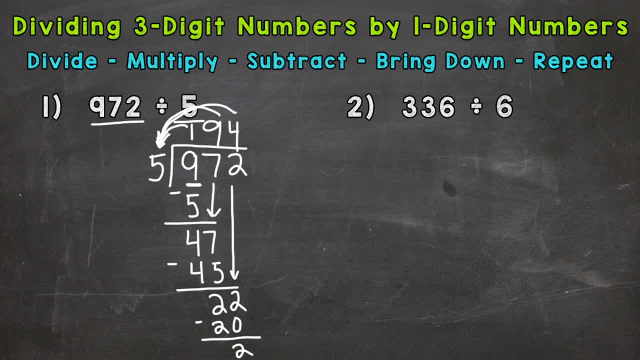 the way over to the ones place, so that 2 down there. that's our remainder. so we have 2 left over. okay, the problem didn't work out to give us a perfect whole number. there we have something left over, so 194 remainder. 2 is our final answer. 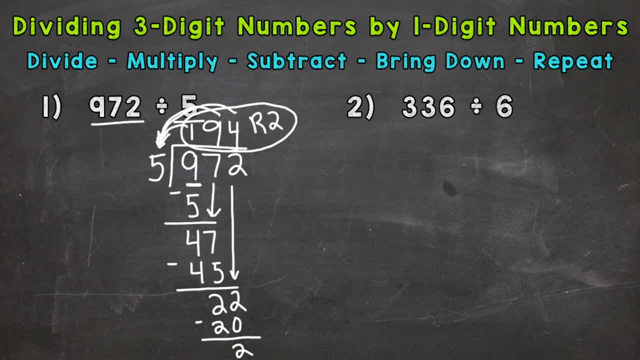 so, again, a lot of steps there, but with the more practice, the more you go through those steps, the easier and more fluid you will get. so on to number 2 and this problem. we're going to use the same process, but it is a little different, and 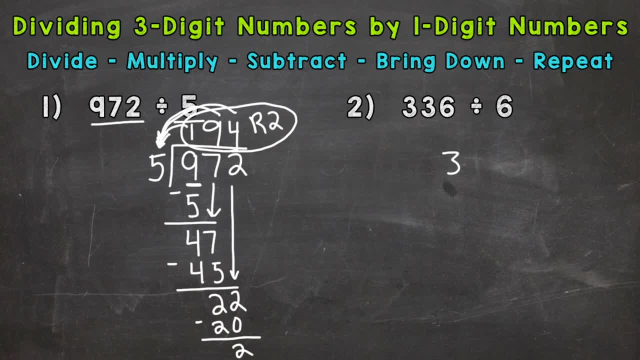 you'll see why here with the first step. so let's set it up: 336 divided by 6. now our first step is divide. so we take a look at our first number here and we have 3 divided by 6. So how many whole groups of six can we pull out of three? Well, we can't do that. 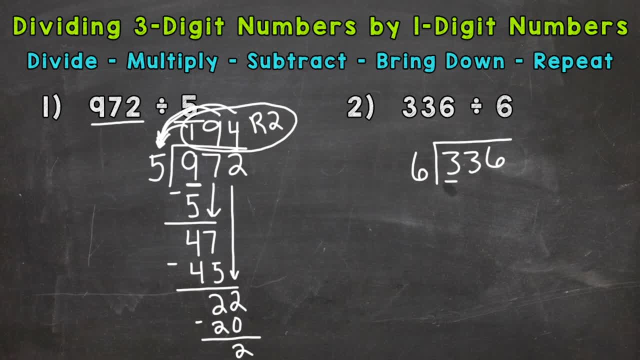 We don't have enough to pull a whole group of six out of three, So we need to take a look at 33. we can look at the next number over and Consider that 33 there, So 33 divided by 6.. So how many whole groups of six out of 33??